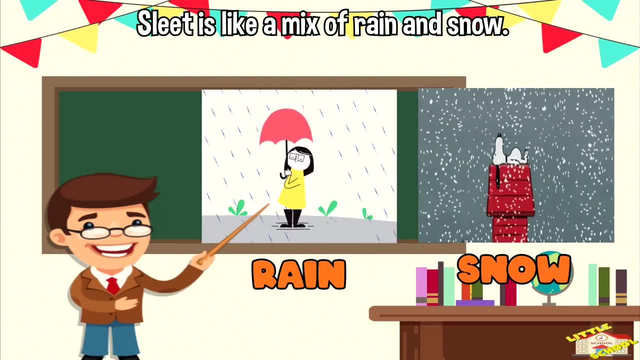 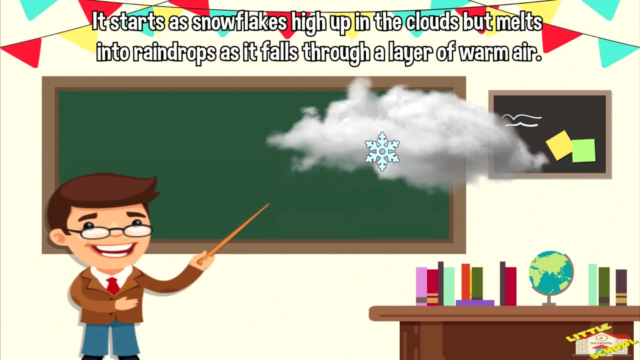 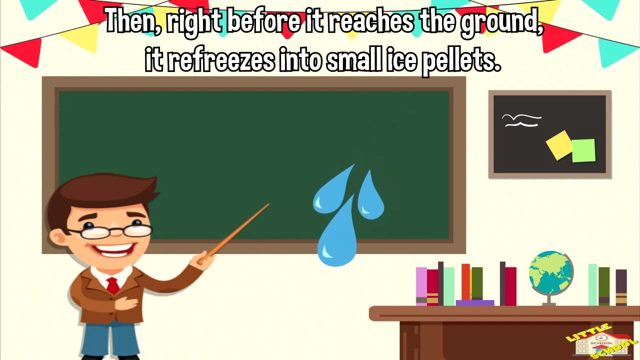 carry rain away from the clouds. a mix of rain and snow. It starts as snowflakes high up in the clouds but melts into raindrops as it falls through a layer of warm air. Then, right before it reaches the ground, it refreezes. 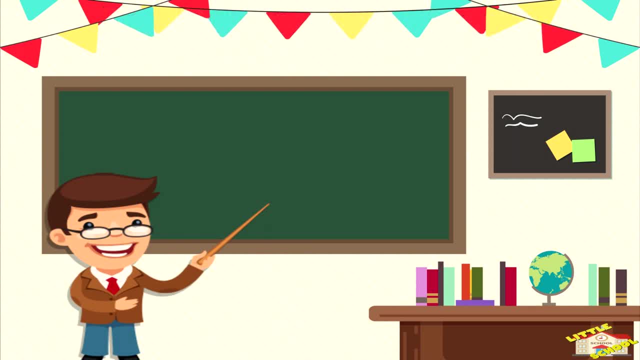 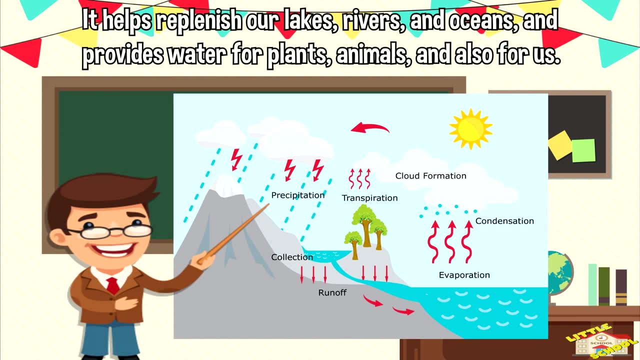 into small ice pellets. Precipitation is an essential part of the water cycle. It helps replenish our lakes, rivers and oceans and provides water for plants and animals, and also for us. Scientists measure how much precipitation fall in different areas using a special tool. 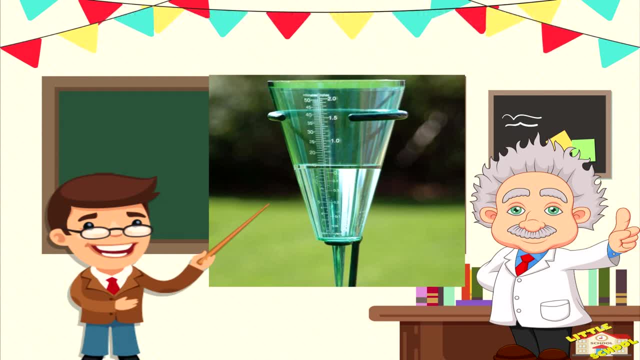 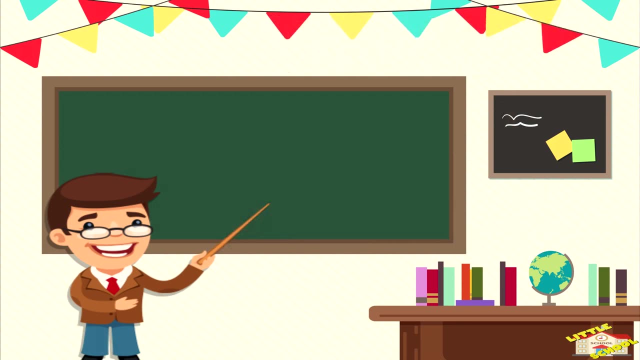 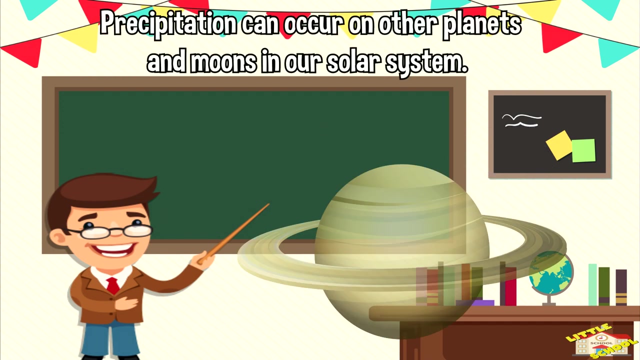 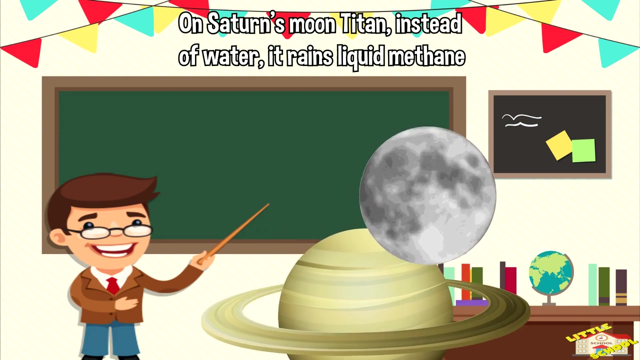 called a rain gauge. It helps us keep track of how much rain we receive per day – both air and air cortisol positive. Closed Rotation. No two snowflakes are exactly alike. Precipitation can occur on other planets and moons in our solar system, For example on Saturn's moon Titan. instead of water, it rains liquid. 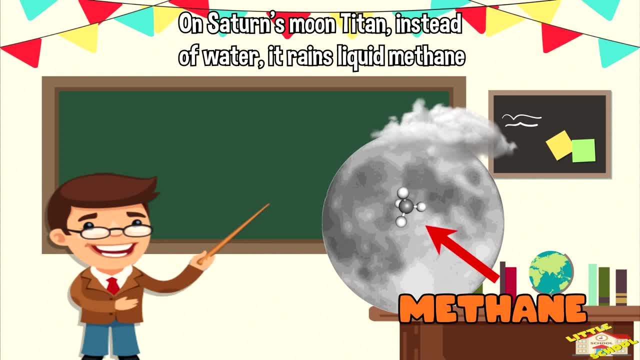 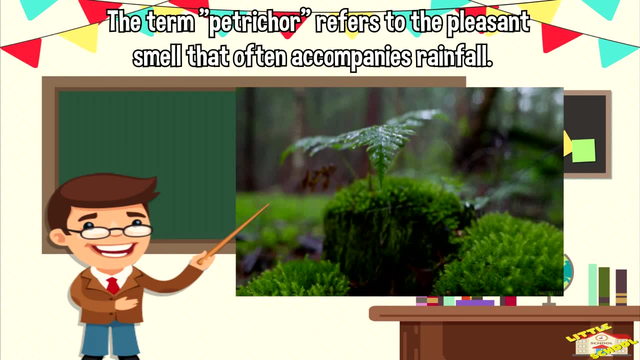 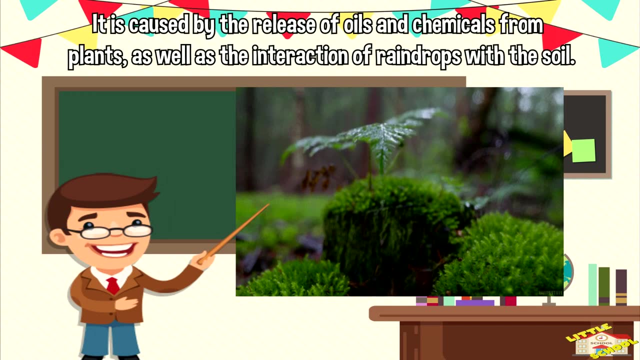 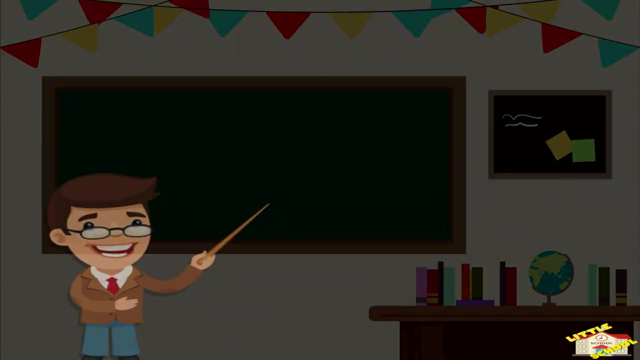 methane Waterhalve म. The term petrichor refers to the pleasant smell that often accompanies rainfall. It is caused by the release of oils and chemicals from plants, as well as the interaction of raindrops with the soil, And that is all for today's video. 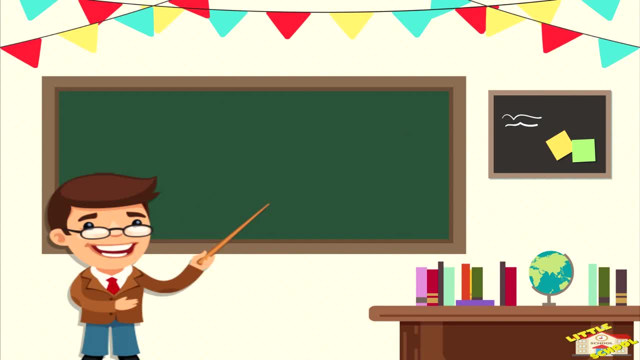 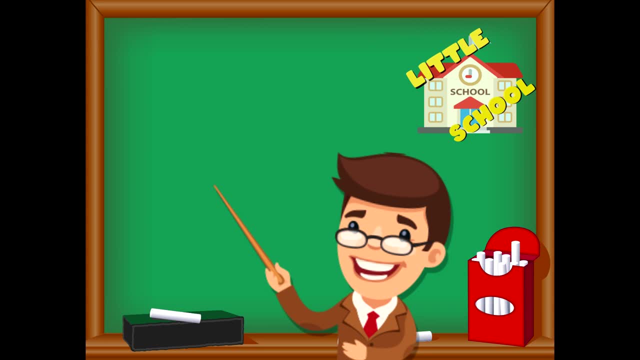 I hope you enjoyed learning about precipitation today. Take care now, bye, bye.